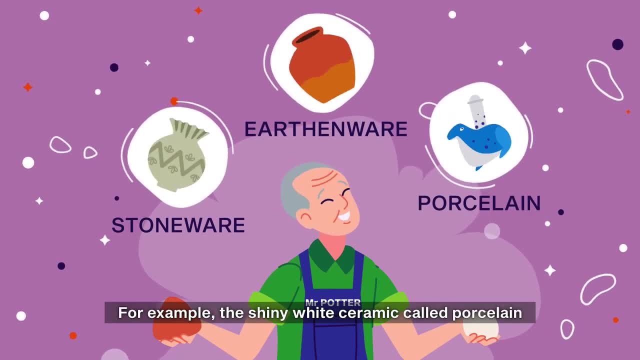 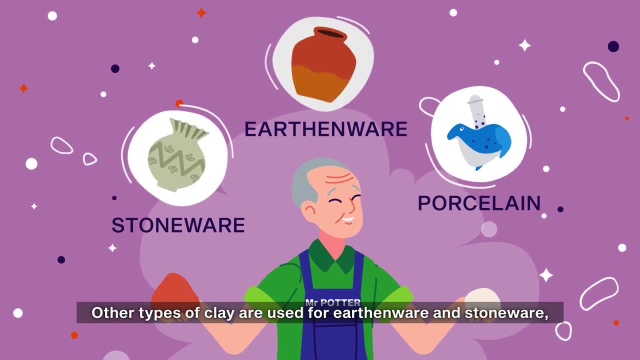 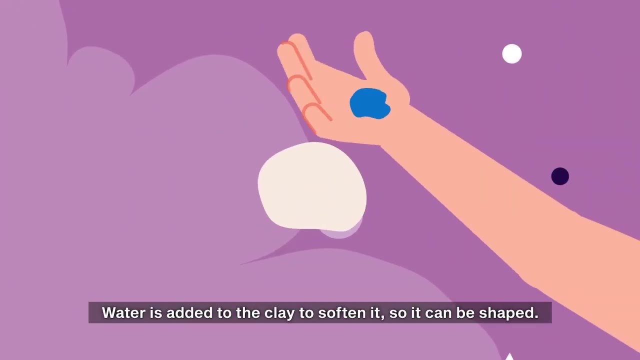 different ceramics. For example, the shiny white ceramic called porcelain is often made using a whitish clay known as kaolin. Other types of clay are used for earthenware and stoneware, which differ in texture and color. Water is added to the clay to soften it so it can be shaped. Can you? 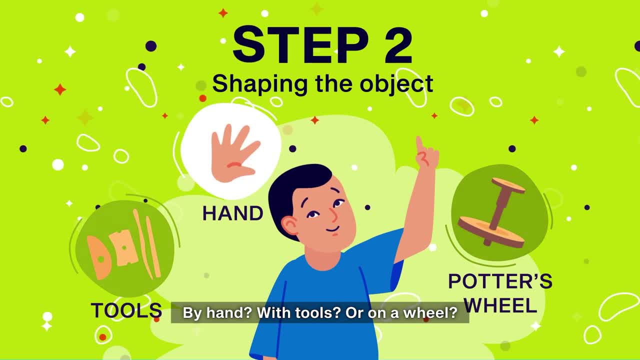 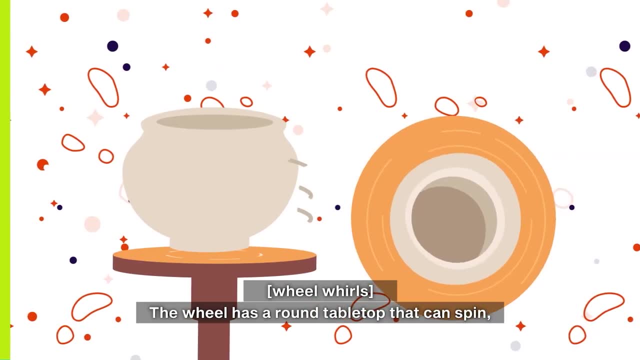 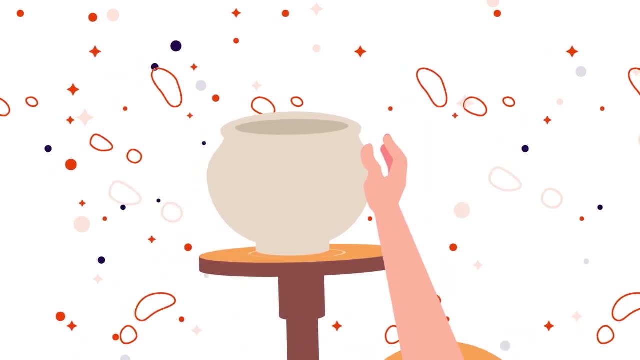 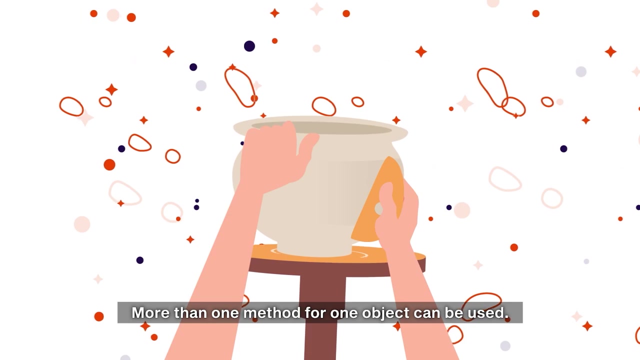 guess how clay is shaped? By hand, with tools or on a wheel? The answer is: all three methods can be used. The wheel has a round tabletop that can spin, so it is good for circular objects like fish tanks. Unusual shapes might need to be shaped by hand. More than one method for one object can be. 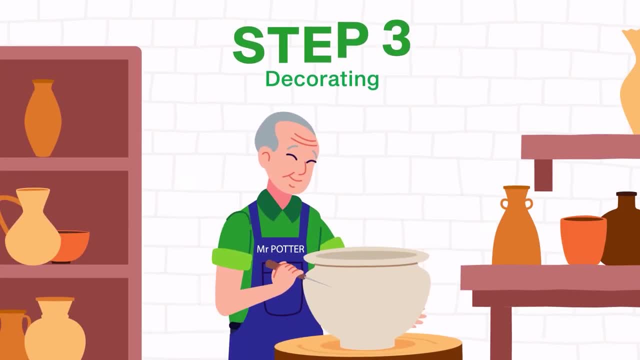 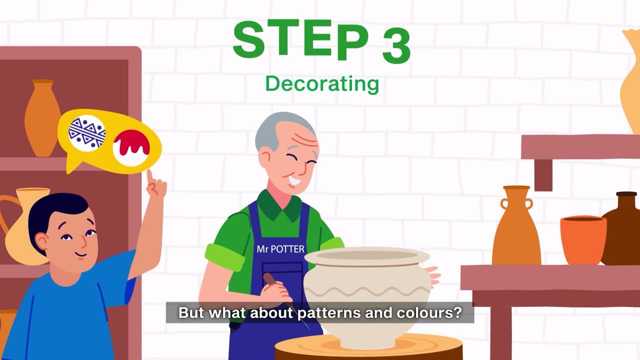 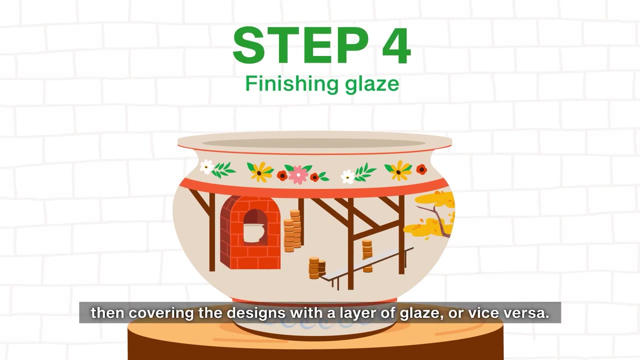 used. Next comes the decorating stage. The potter uses tools to add details and decorations. But what about patterns and colors? Those can be done by painting the surface of an object, then covering the designs with a layer of glaze, or vice versa, The glaze- 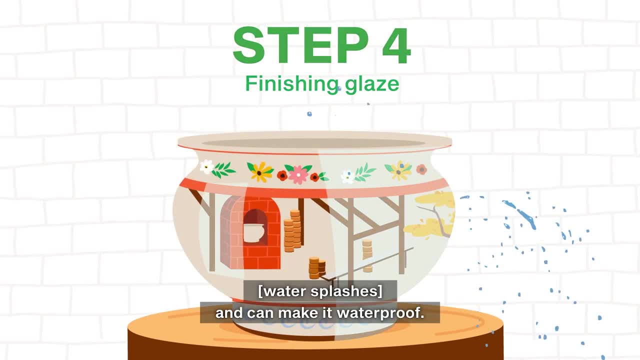 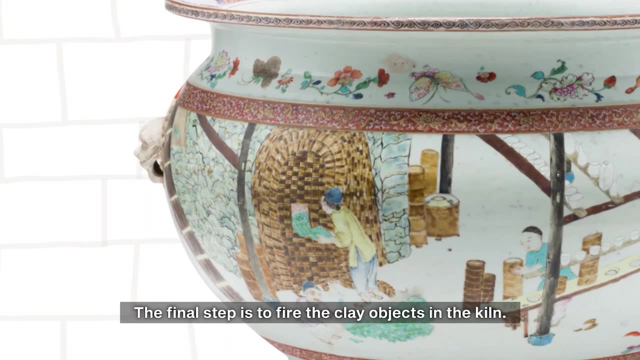 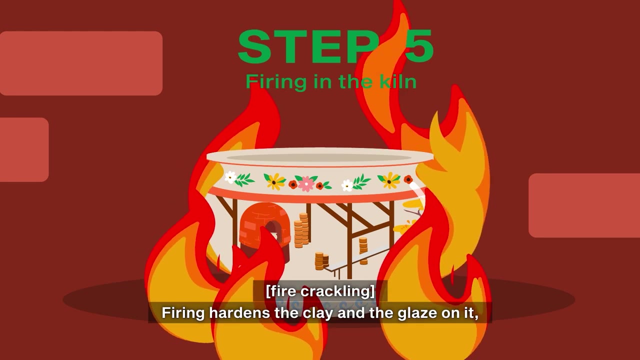 gives the object a glassy surface and can make it waterproof. Look, here's a potter glazing on our fish tank. The final step is to fire the clay objects in the kiln. A kiln is a large oven used to bake clay. Firing hardens the clay and the glaze on it, making it stronger and more durable. 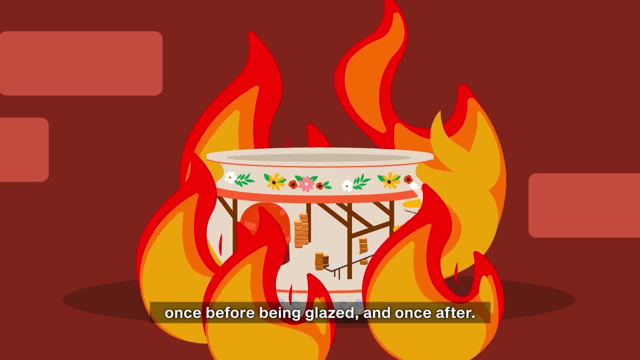 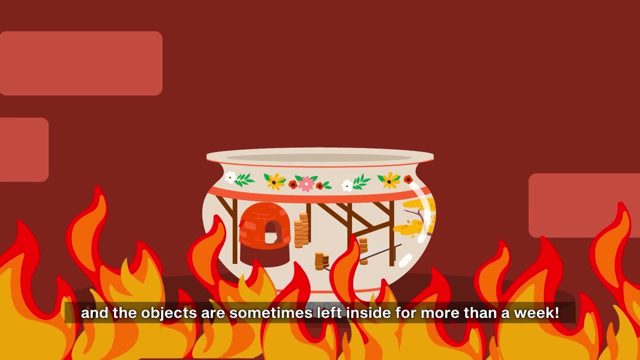 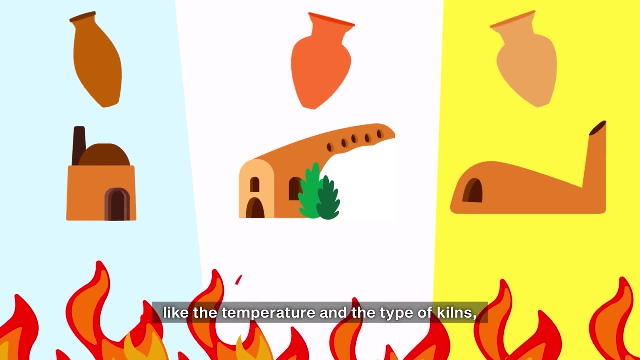 Some ceramics are fired twice: once before being glazed and once after. A kiln can be heated to over a thousand degrees Celsius and the objects are sometimes left inside for more than a week. Different firing conditions, like the temperature and the type of kilns 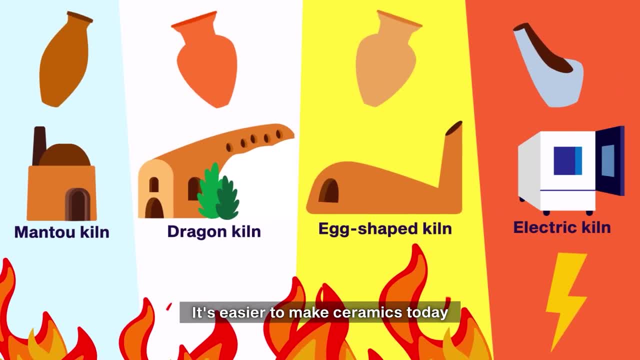 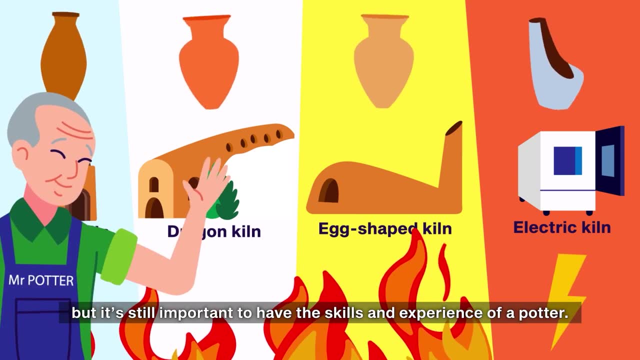 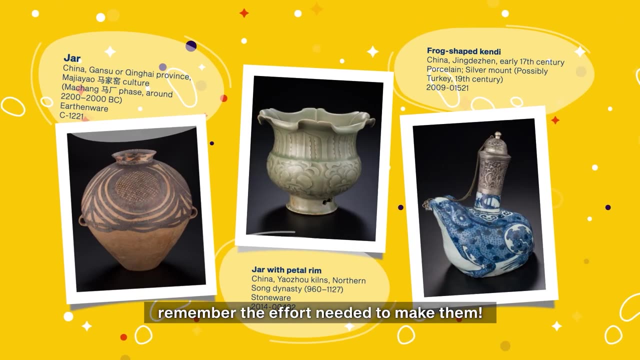 can change how the final ceramic looks. It's easier to make ceramics today with the help of machines and electric kilns, but it's still important to have the skills and experience of a fireman. So next time you see ceramics, remember the effort needed to make them. 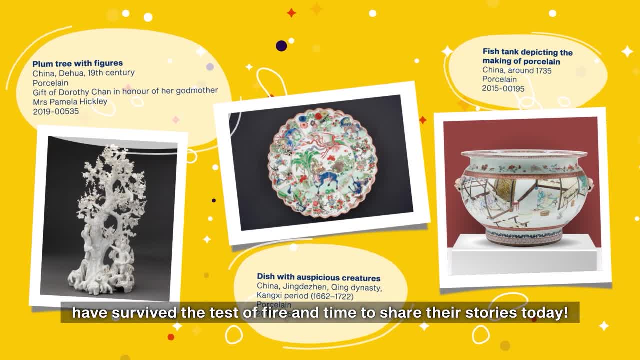 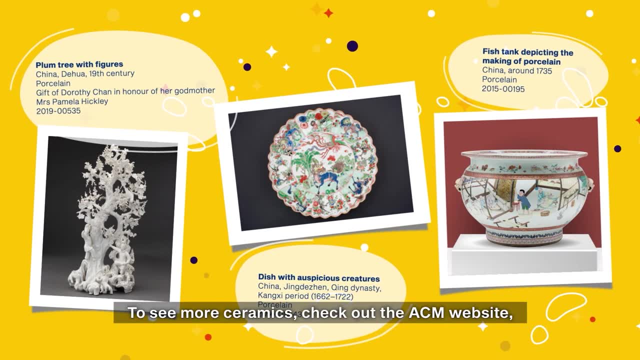 Old ones like my home have survived the test of fire and time to share their stories today. To see more ceramics, check out the ACM website or come visit us at ACM today.